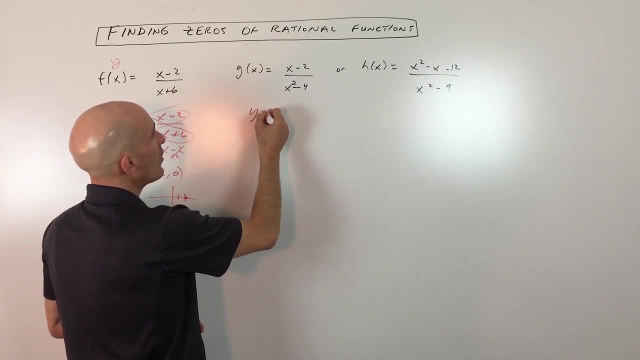 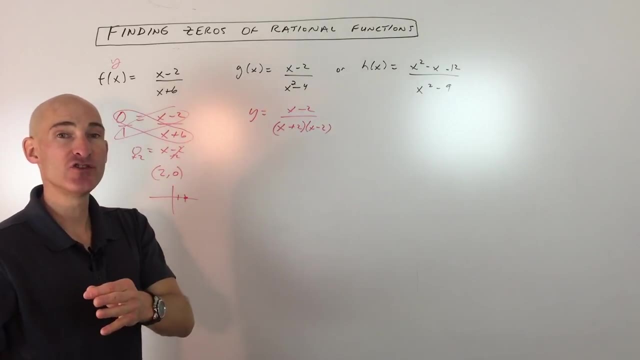 Okay, now for the second example. what you want to do for this one is you want to factor the numerator and the denominator as much as you can, and the reason is is because if you have a factor in the numerator, that cancels with a factor in the denominator. 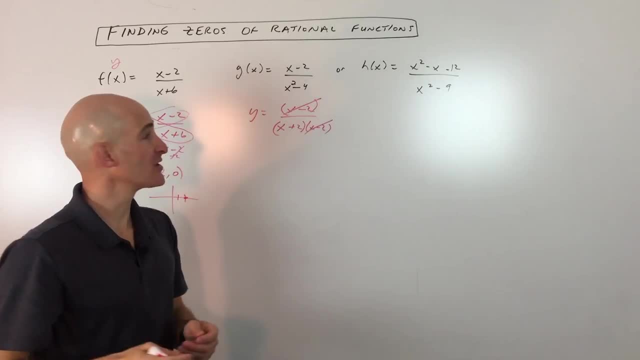 like you see here, x minus two, you're not going to actually have a point on your graph at that point, because what happens is it's actually a hole in the graph, or what they call a removable discontinuity. So, in all practical, for all practical purposes, 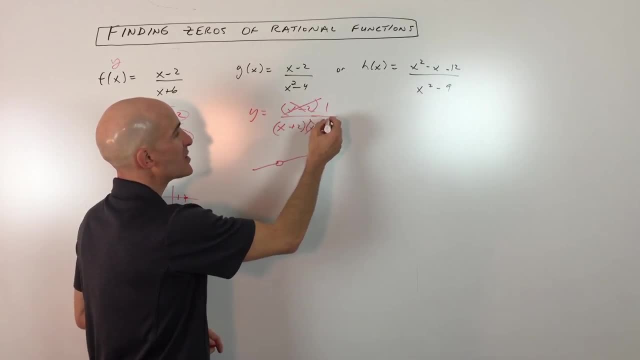 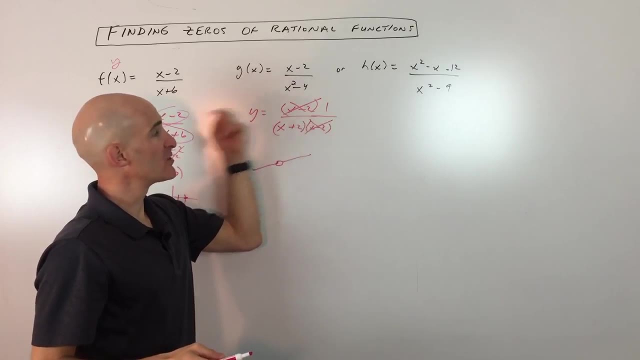 these factors are canceling one another out and your basic equation now is going to look like one over x plus two. So here you can see that if you try to set the numerator to zero, like we did in this previous example, you can't really set a constant to zero. 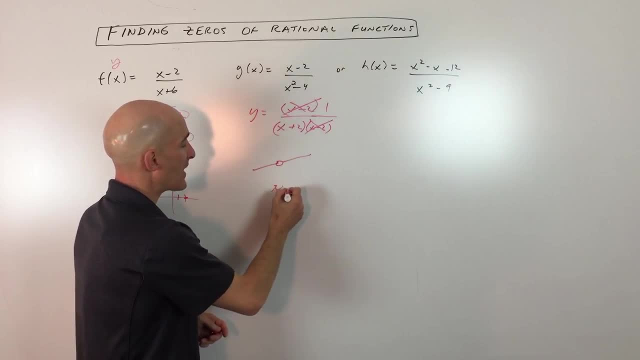 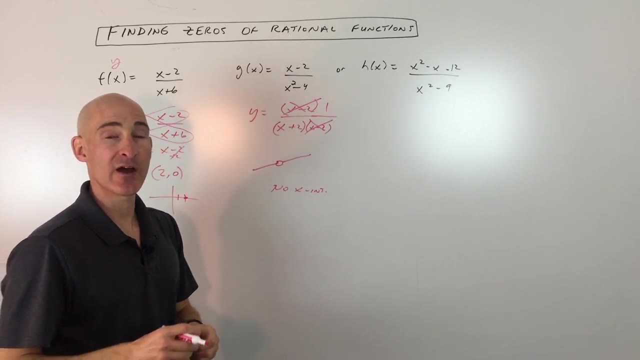 So what this means is that there's no zeros, there's no x-intercepts for this particular graph. Okay, there's going to be a hole, and I talked about that in another video. you can check that out. on Graphing Rational Functions: 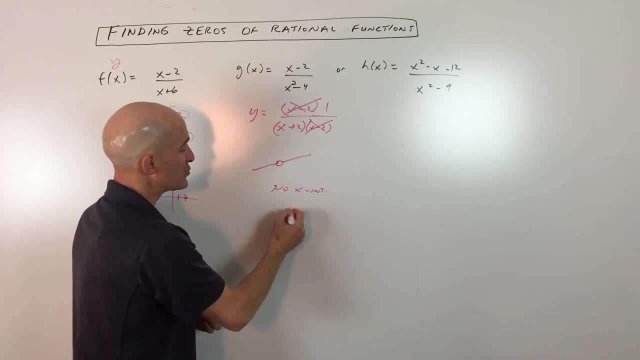 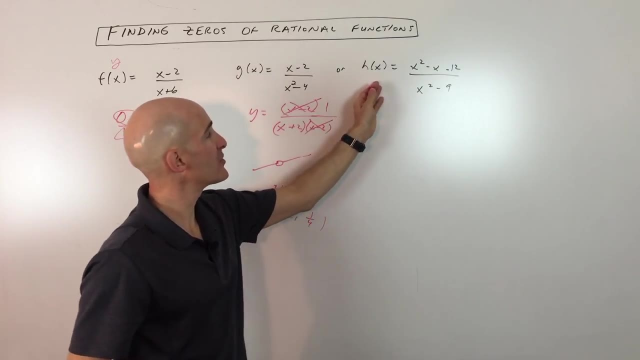 but the way you would locate the hole is the hole would be at two comma. now if you put two into what's left over here, that's going to be one fourth, But in this case we're just talking about the zeros. So let's look at the third example. 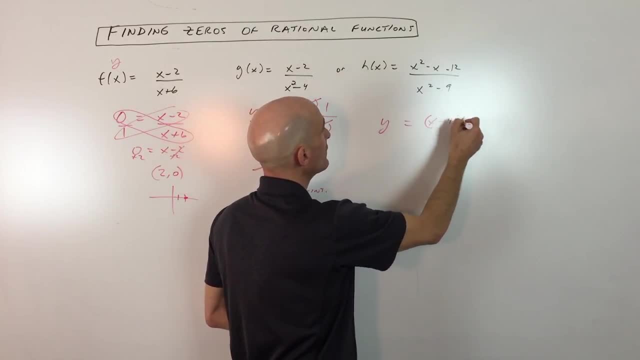 Same thing. you want to factor the numerator- okay, x minus four, x minus two, x plus three. and you want to factor the denominator: it's the difference of two squares, x minus three, x plus three. again, notice that these x plus threes are canceling. 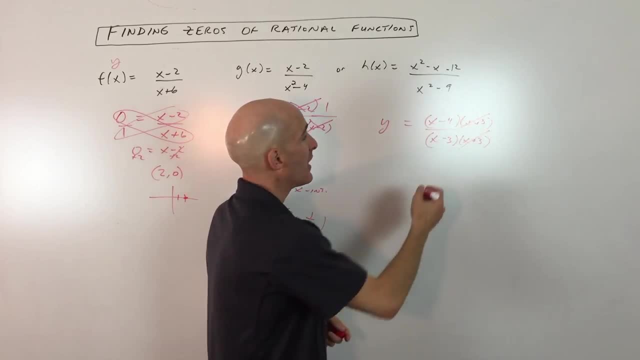 so we're not going to have a zero at negative three if we set the numerator to zero. we're just going to have an x-intercept at four or a zero at four. so this graph's going to cross at four comma zero, right there. 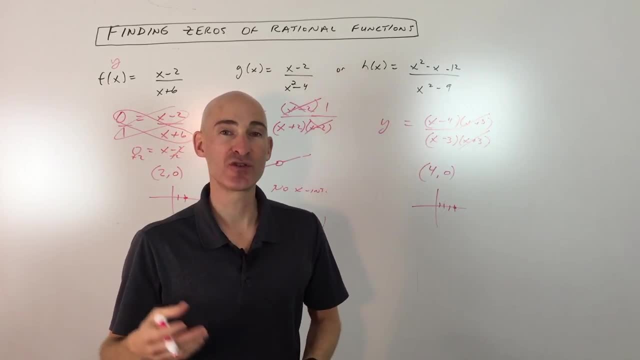 So I hope this helped you understand how to find the x-intercepts or the zeros when you're graphing rational functions. Subscribe to the channel. check out some more videos on Mario's Math Tutoring YouTube channel and I look forward to helping you in the future videos. I'll talk to you soon.